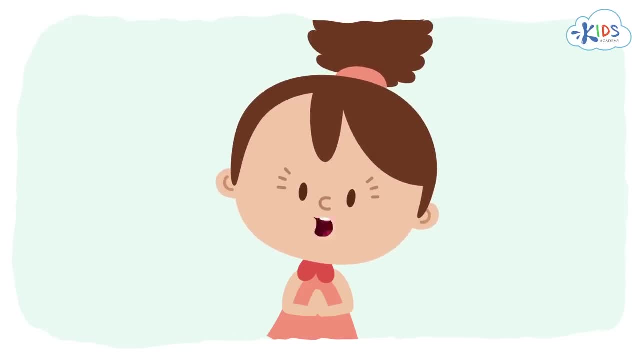 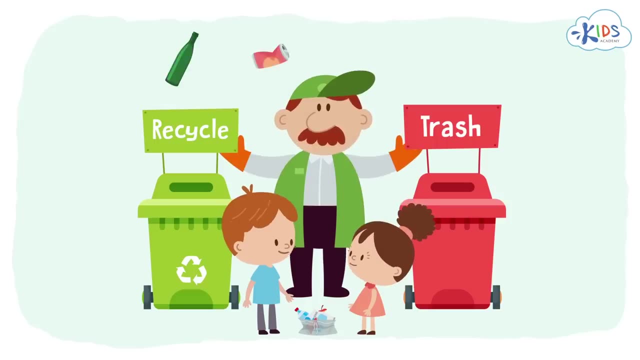 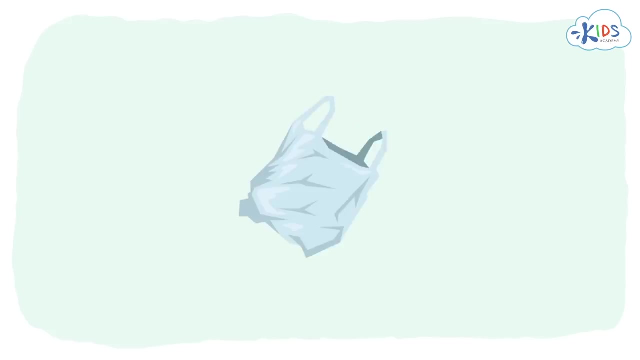 That's recycling. Wow, That's amazing. Well, how can we recycle? You can start by putting all of the recyclable trash into the correct bin. Remember: only glass, metal, plastic and paper can be recycled. I think we need some help. 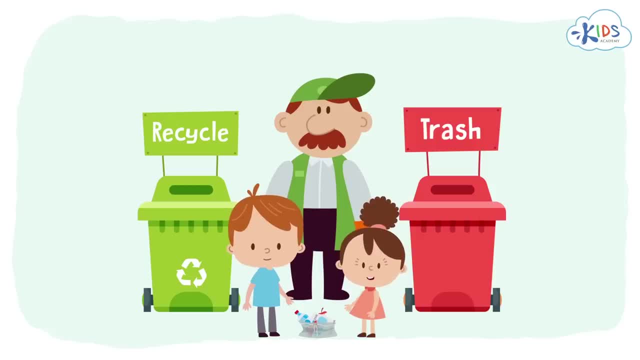 Can you help us sort the trash? Great, Let's clean up. Where should we put this plastic water bottle? In the trash bin Or the recycling bin? You're right, Let's toss it in the recycling bin. Hmm, What about this apple core? 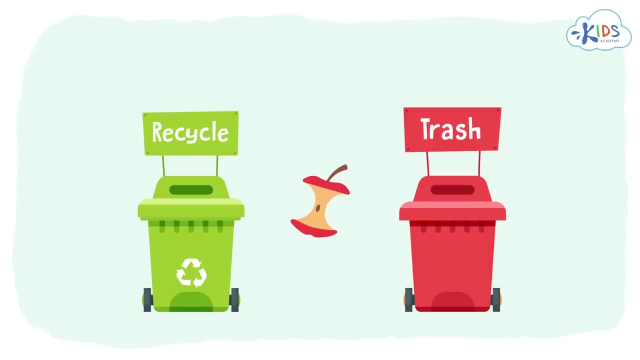 Can we recycle it? No Food goes to the trash bin. Do you know where this soda can goes? Yes, We can recycle metal cans. Let's keep going. We have an egg shell, an empty glass bottle, an old magazine. 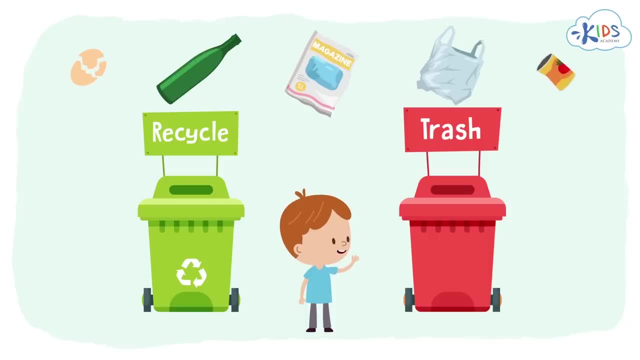 a plastic bag and a metal can. Can you help us sort them? We will give you some time to think, But if you need more time, you can pause the video and answer when you are ready. You already know that we can recycle glass, metal, plastic and paper. 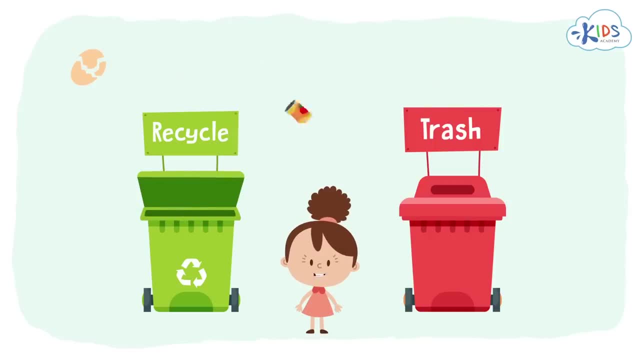 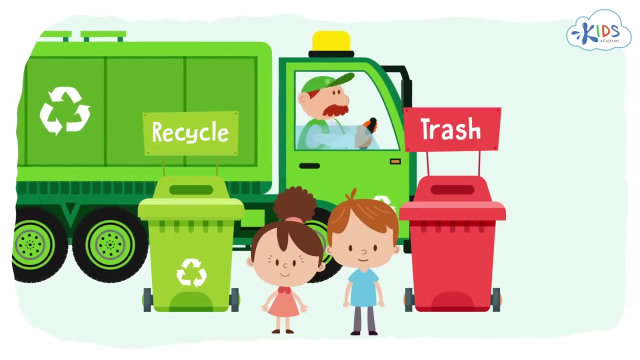 That's why these things should go into the recycling bin. Can we recycle food? No, The egg shell goes to the trash bin. Wow, You two did a great job. Thanks to you, Mr Sammy, And thanks to you, Good-bye. 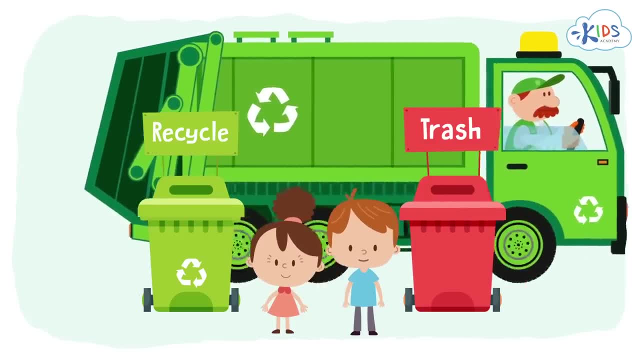 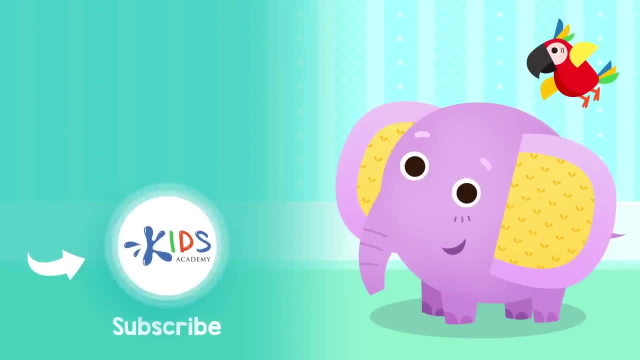 Good-bye, Good-bye.